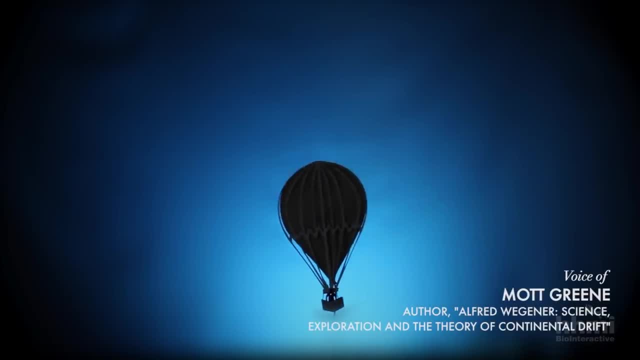 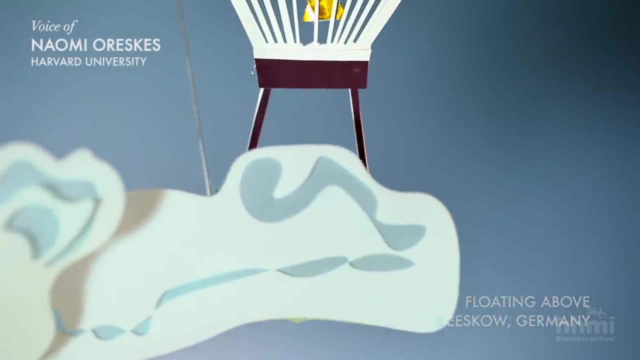 Getting into a balloon and going up into the air for a meteorologist is like getting into a boat and going out on the ocean for an oceanographer. He goes up in a balloon because he wants to take measurements of the atmosphere. He's not the Wizard of Oz, He's a scientist doing science. 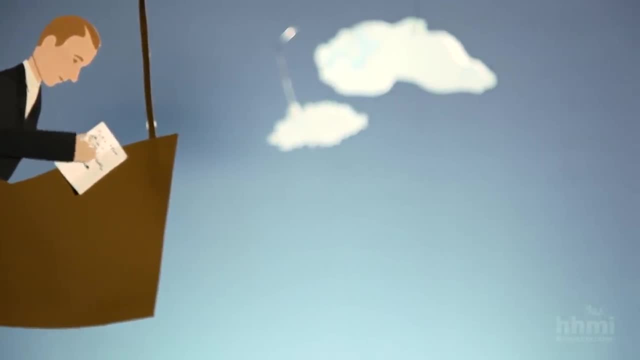 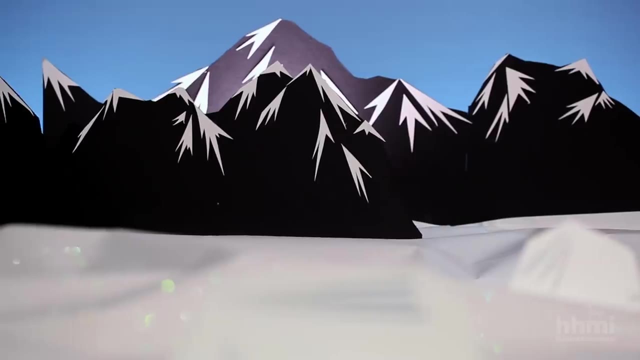 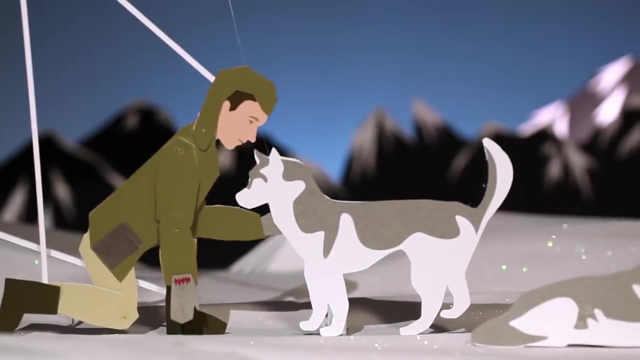 Wegener flew as much and as often as he could. he wants to write the best book on the physics of the atmosphere, and no one had ever studied the atmosphere in the high Arctic before. This is a time in history when one of the most exciting things you can do as a scientist- 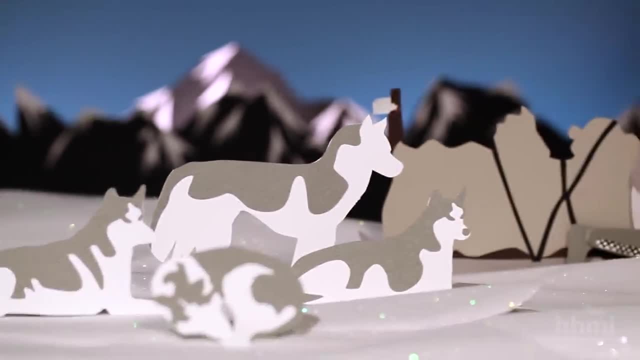 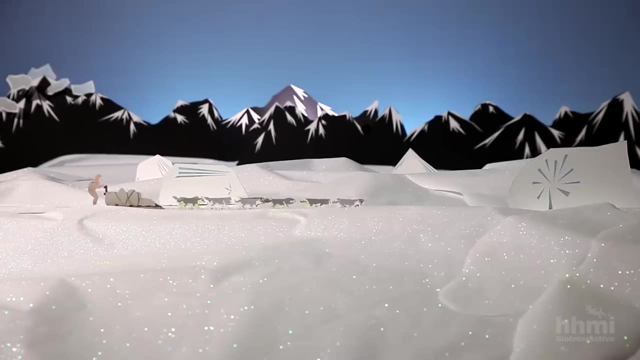 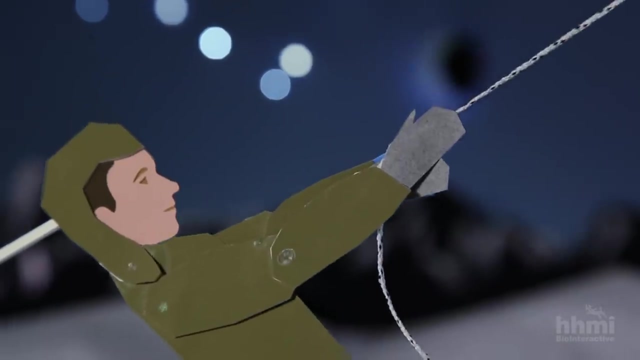 is to go on an Arctic expedition. It was adventure travel of a North Pole, South Pole kind. Wegener is out there. Wegener is out there. Wegener is out there in the winter night taking these huge box kites and attaching recording instruments to them. 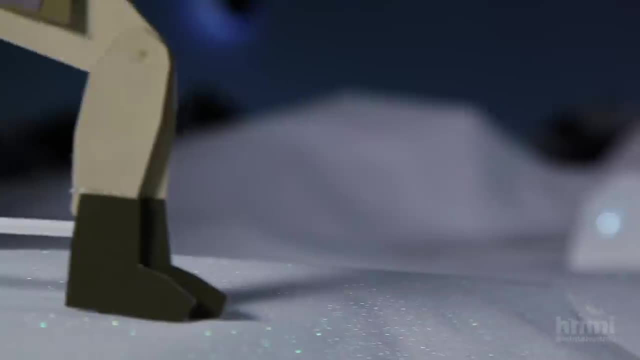 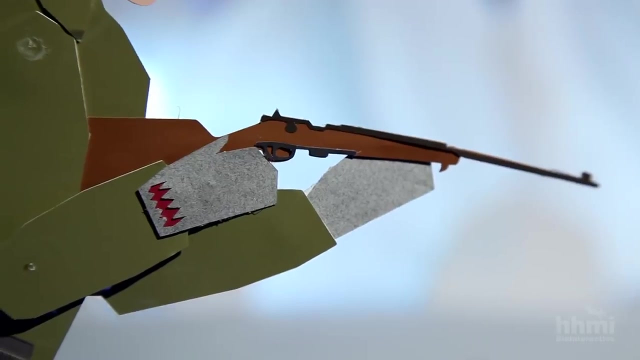 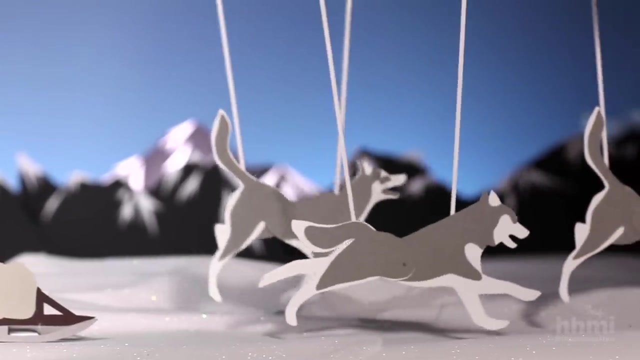 and then winching them back down to get his instruments back. Nobody ever said that Arctic exploration was a picnic. Wegener had to learn how to hunt seals, how to drive a dog sled, how to travel on ice without being swept into open water. 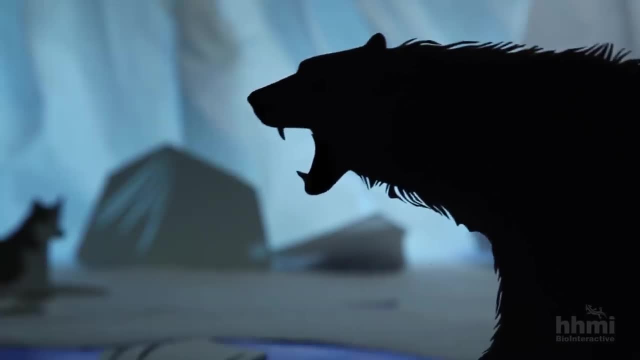 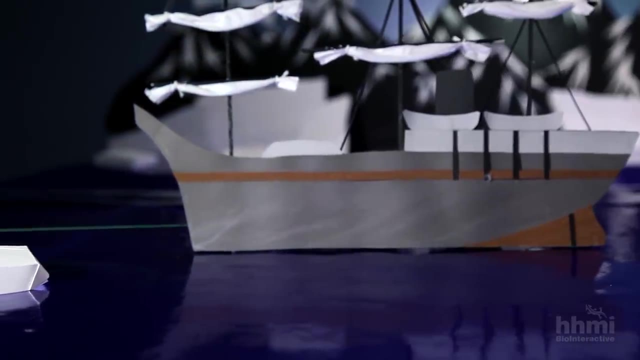 how to protect your dogs from polar bears, how to keep them from being eaten by the polar bears. He was a scientist who was very familiar with the icebergs. The travel in Greenland, his time with icebergs, The way in which the ice flows, form jigsaw puzzle pieces. 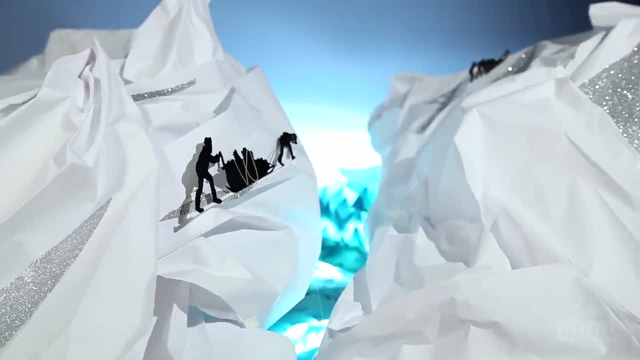 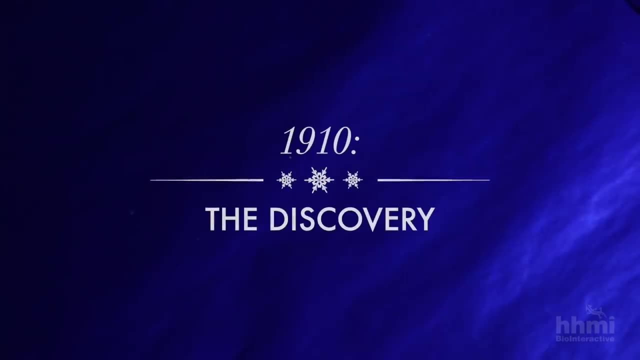 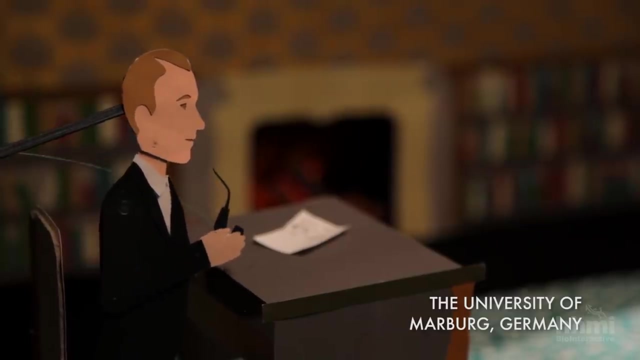 The way the ice cap splits apart and fissures. All of this was part of his imagination when he made his discovery of continental drift. I wouldn't really call it a discovery. What he really had was an idea. He went to his office and his office mate said: 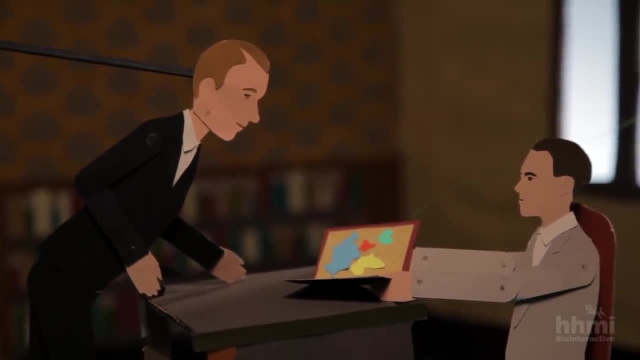 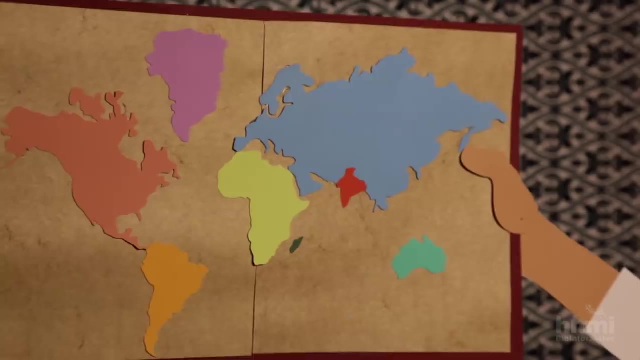 look at this beautiful atlas my parents gave me for Christmas And he wrote to his fiancée: did you ever notice how South America fits into Africa? Let me pause and say there isn't a child on Earth over the age of 12. 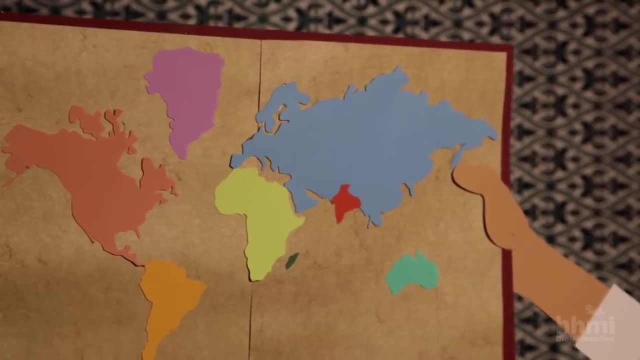 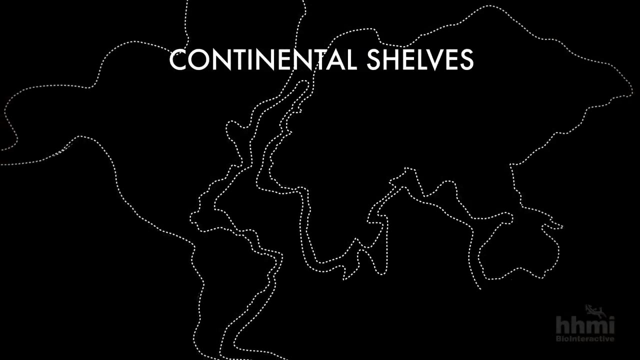 who hasn't had the same thought. right, You can see it. What was different about what Wegener saw? There were lines on the map that represented depths under the water, and they're exactly the same shape. That means that this is part of the structure of the Earth. 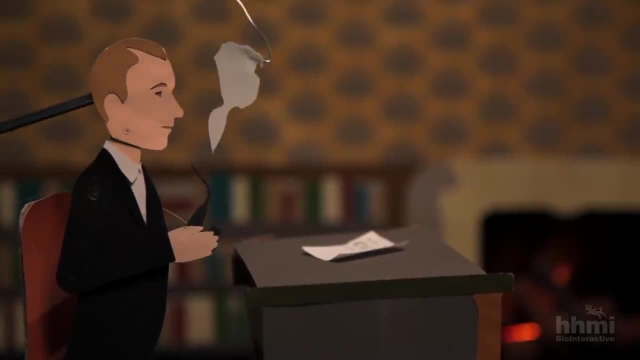 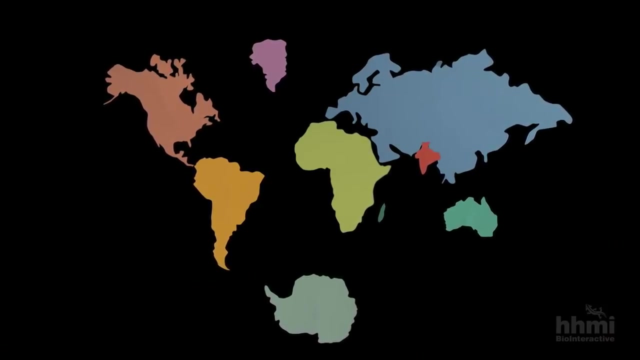 How did that come about? Maybe the continents drifted apart? It was radical because it was new. The Americans say the continents are fixed. Europeans think they move, but they think they move up and down. And Wegener says: you're all wrong. 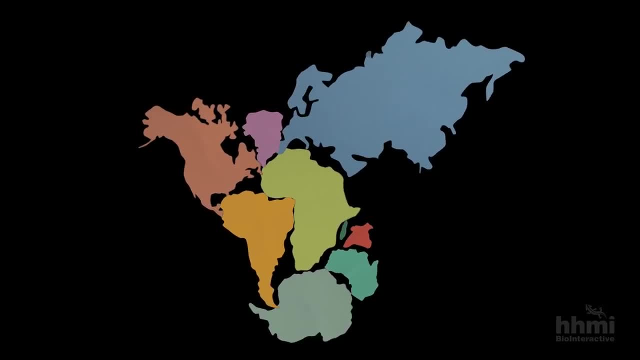 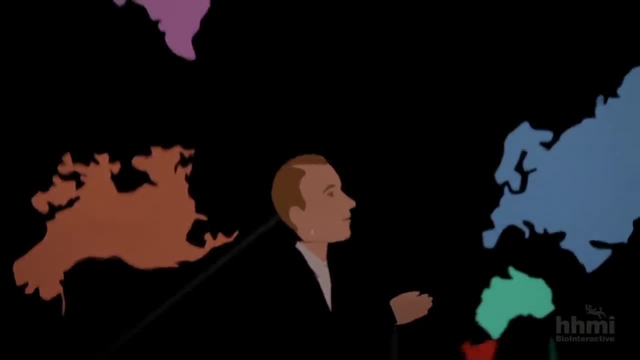 Yes, they move, but they move horizontally, not vertically. He would write a paper in 1912, and he said: I think everybody will really be happy. And of course everyone wasn't really happy. Everyone became very unhappy. 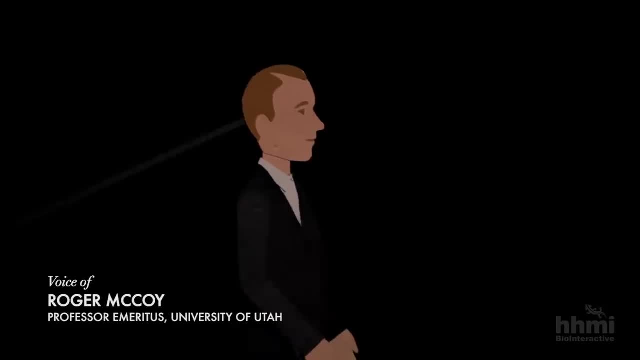 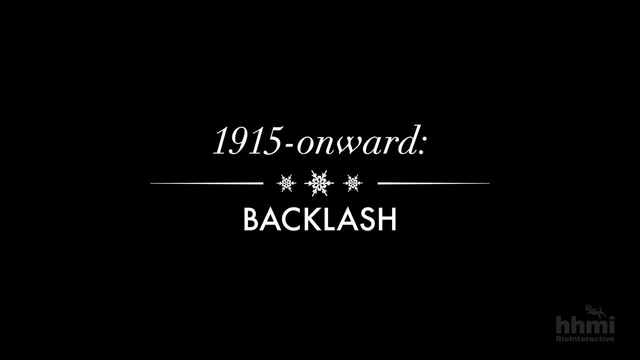 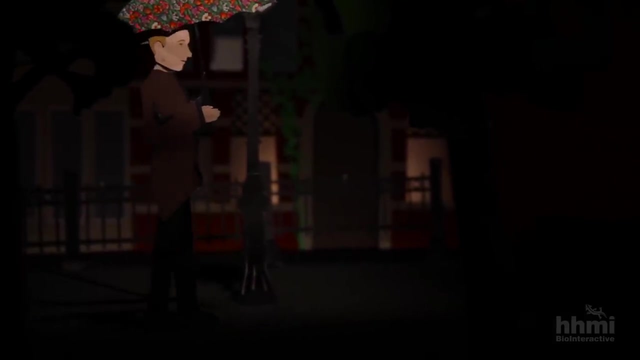 There was an almost universal rejection of his theories to begin with. Here's the problem: Scientists are very suspicious of fundamental novelty. He was regarded as an outsider by the geoscience community because he had no academic background. He had no academic credentials in that field. 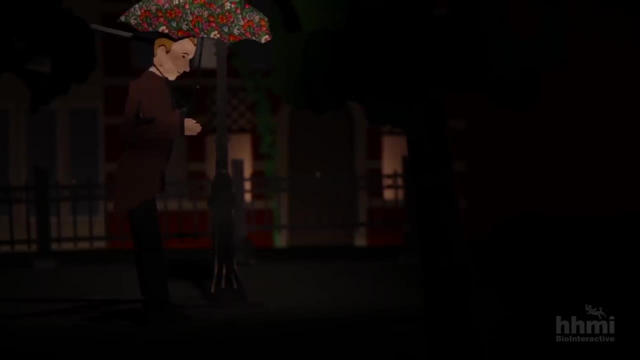 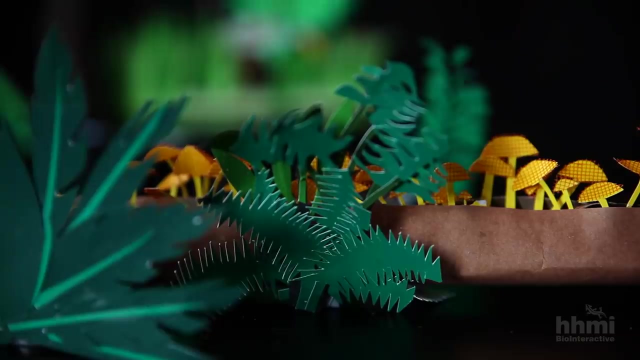 and so he was not considered qualified to make any statements in that field. What he was doing that was so different, though, was drawing together multiple lines of evidence, not just geology, but vegetation and paleontology. The botanical people responded very positively. 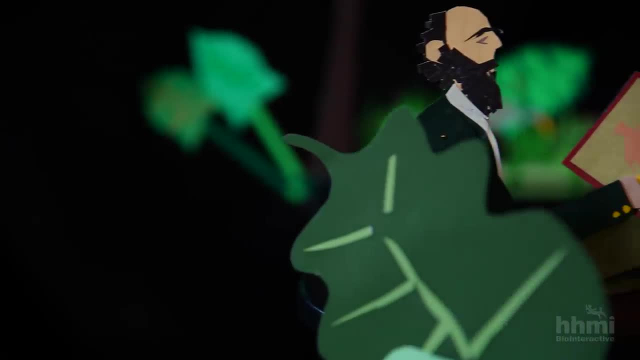 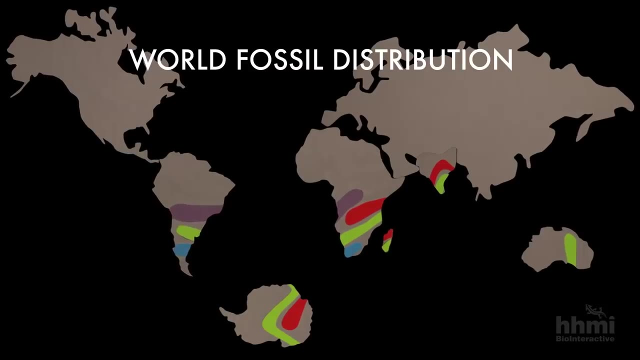 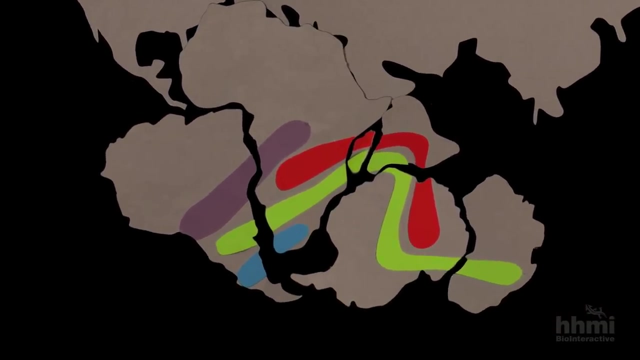 because it explained the distribution of plants and animals over the world. In different places on Earth, you saw virtually the same fossils. the stratigraphic columns were extremely similar as well, And Wegener's idea, his big idea, was: you could explain all of those things if the continents had moved. 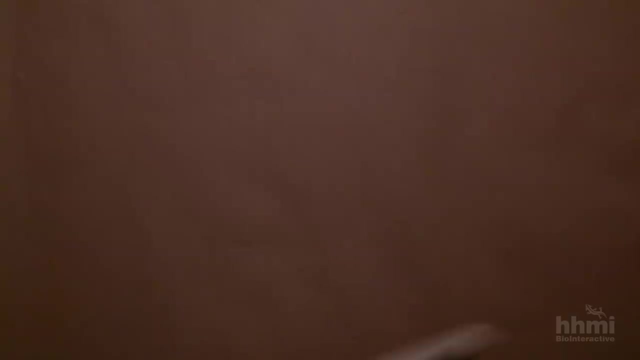 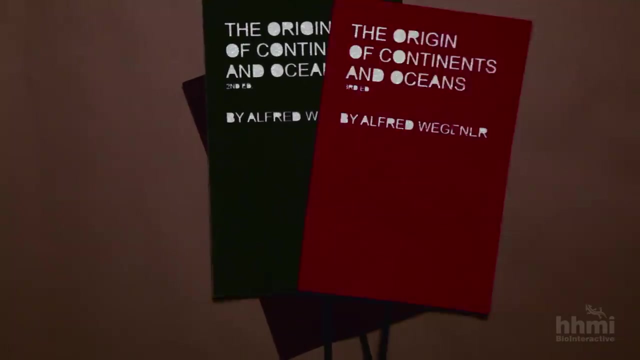 So he would write a book in 1915. People said, well, this is wrong and that's wrong. And then he wrote another book in 1920. He comes up with the name Pangea, And then he wrote another one in 1922. 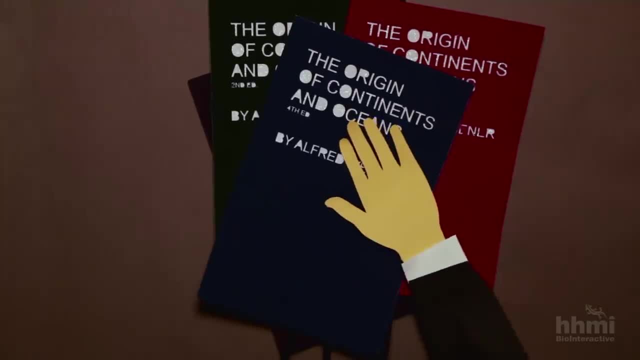 And he kept fixing it and fixing it, and fixing it. It's one thing to think of an idea and it's another thing to work it out for 20 or 30 years. It's one thing to think of an idea and it's another thing to work it out for 20 or 30 years. 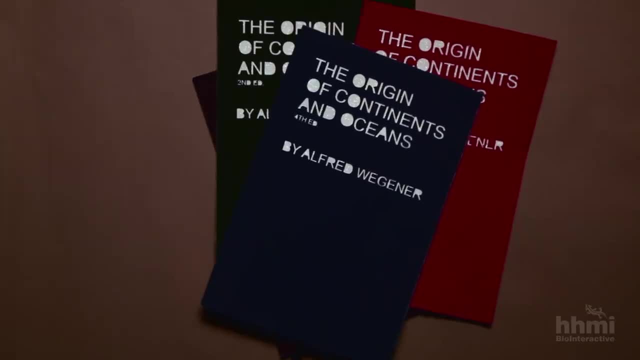 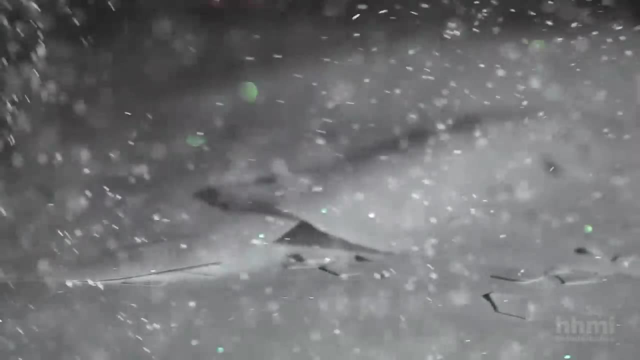 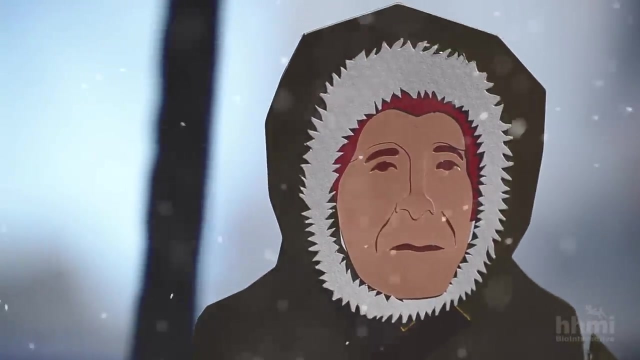 That book's still available on Amazon. Continental drift was something he was interested in, but it was never the focus of his scientific life. The Arctic pulled him back in. He was really too old, almost 50 years old. He landed there with 98 tons of equipment. 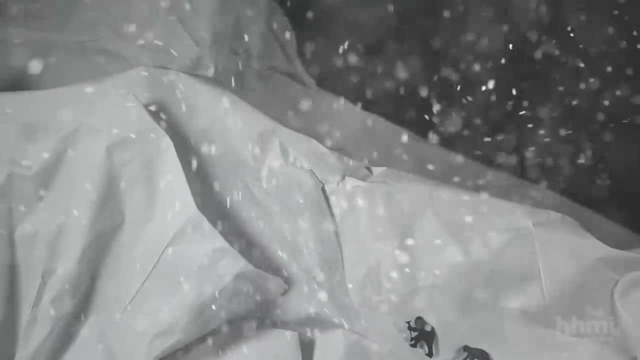 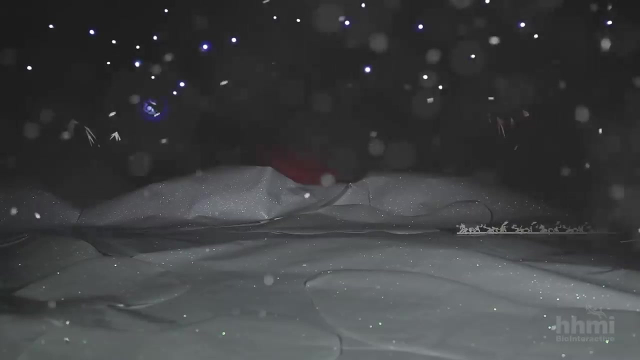 And from the beginning things didn't go well. They had many things go wrong. The base in the middle of the Arctic, the ice in the middle of the ice cap, did not have enough food And he said: this is my responsibility to resupply. 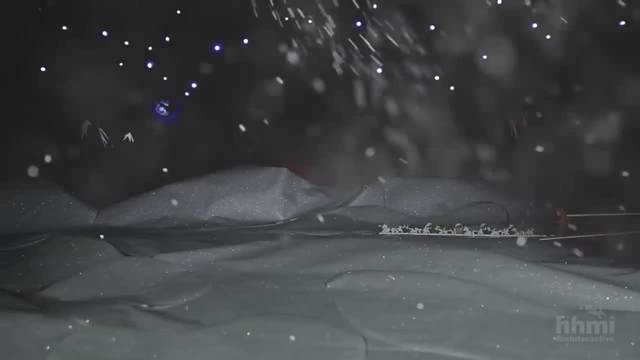 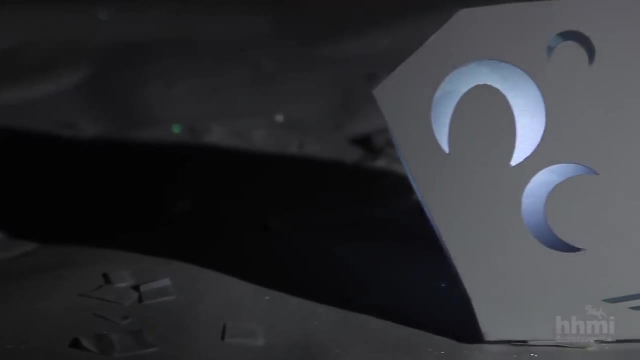 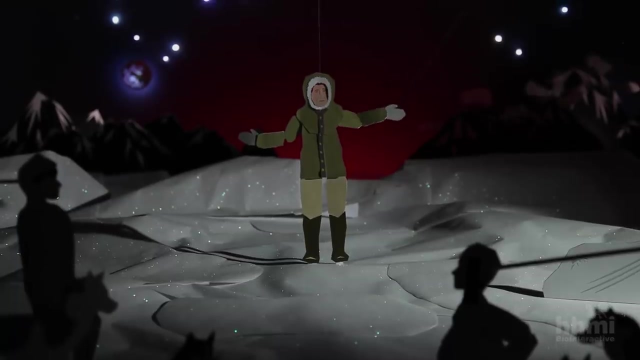 And he got several sleds together. It's the worst conditions you can possibly imagine. His companions wanted to give up And at twilight Wegener said let's go for a walk. And he took them out and pointed to the ice and pointed to the sky and said: 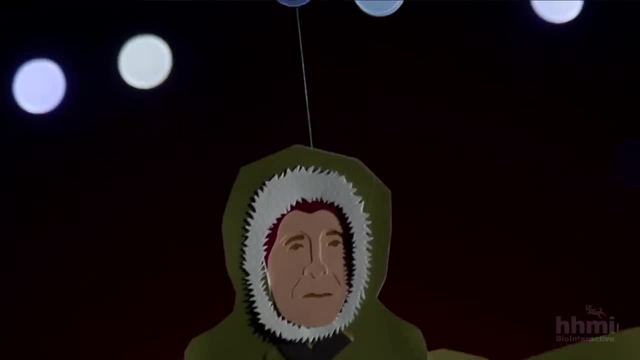 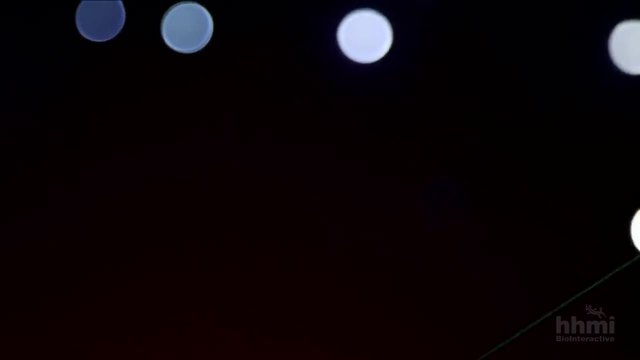 we're trying to find out how all this works. It doesn't matter whether we live or die. The important thing is that the work go on, And I guess that's why I love Alfred Wegener, because it's not really about himself. 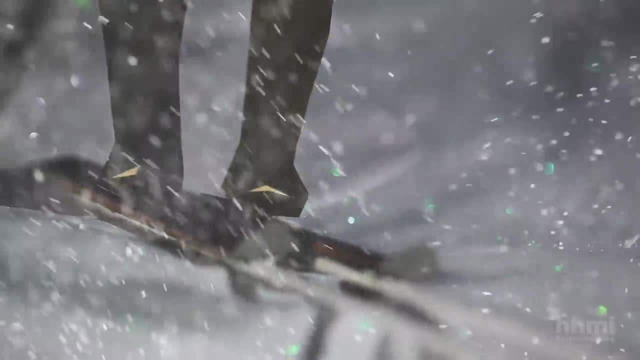 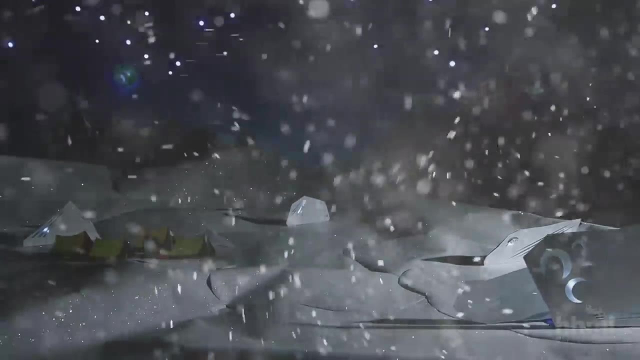 It's that he believes in science, a kind of great metaphorical expedition. At the end of all this they were able to supply the station at the middle of the ice, And then they got there and there wasn't enough food to last the winter for all of them. 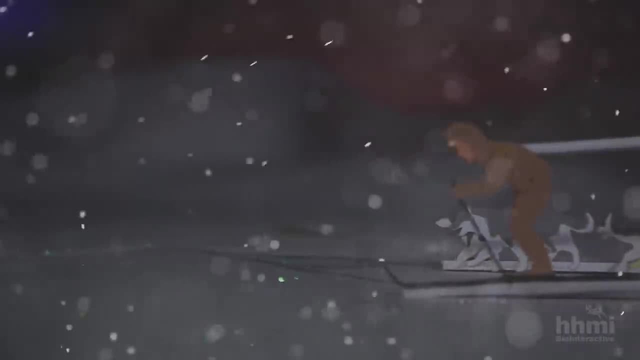 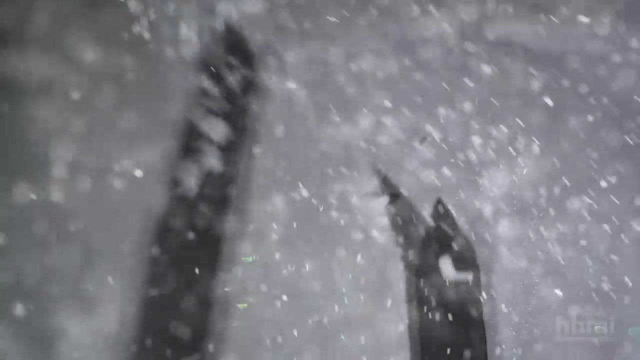 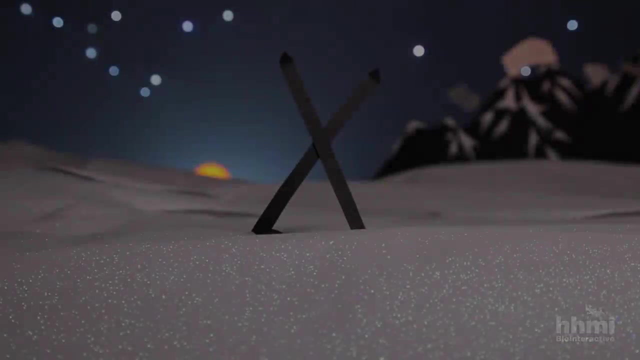 Wegener said I'm going to go back to the coast. He didn't like to ride on the dog sled, He liked to ski next to the dogs. He had a heart attack and died. He's still there. The German government wanted to bring him back for a big funeral.